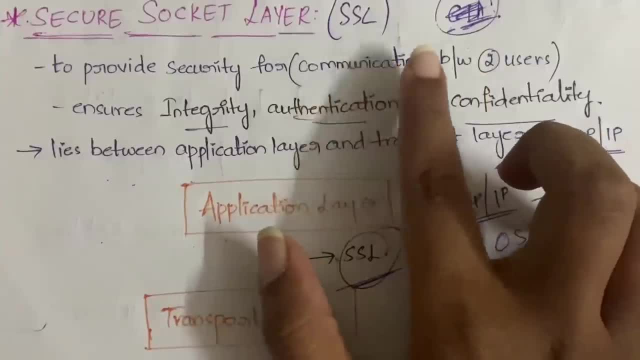 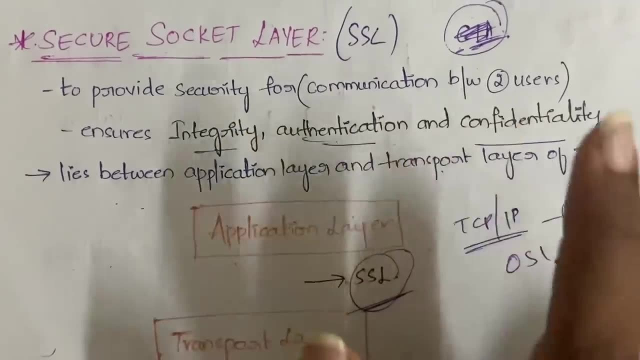 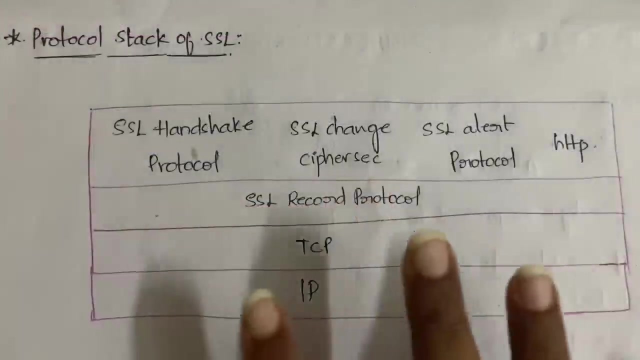 two users, when two users are communicating with each other. in order to provide security to the users, we use this ssl protocol and it ensures for integrity, authentication and confidentiality of the message. got it. now let us see what are the different protocols we have in this ssl. this is the protocol stack of the ssl. basically, these are the protocols. 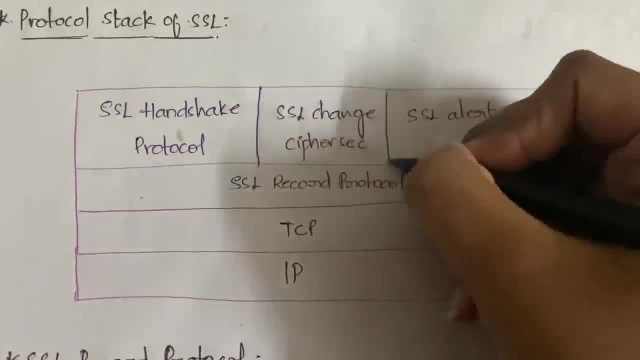 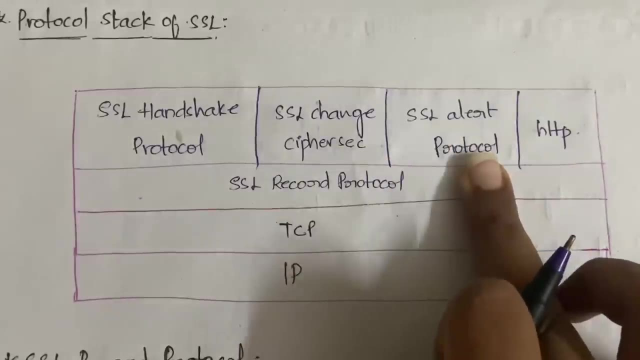 we have in this ssl protocol. so this is the protocol stack of the ssl. basically these are which we have in ssl. uh, so actually there is separation between them. i forgot to draw. so we have handshare protocol, change ssl, change ciphersec protocol. we have ssl alert protocol. 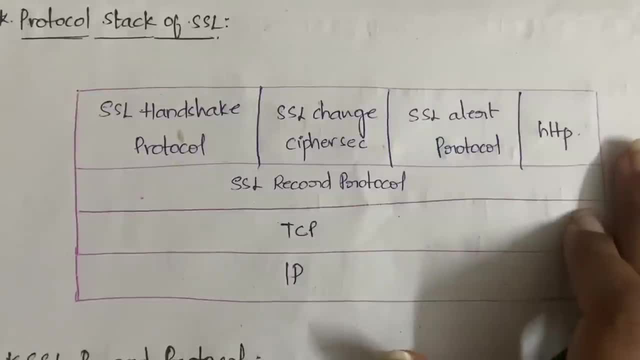 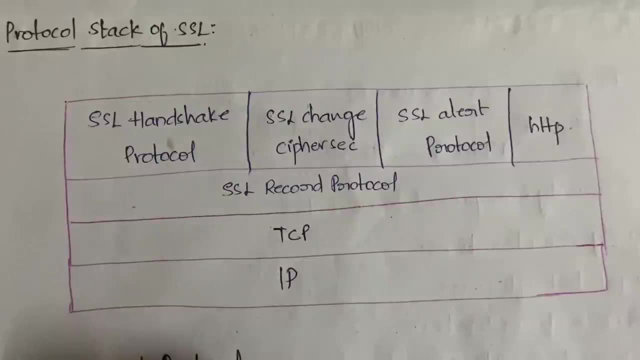 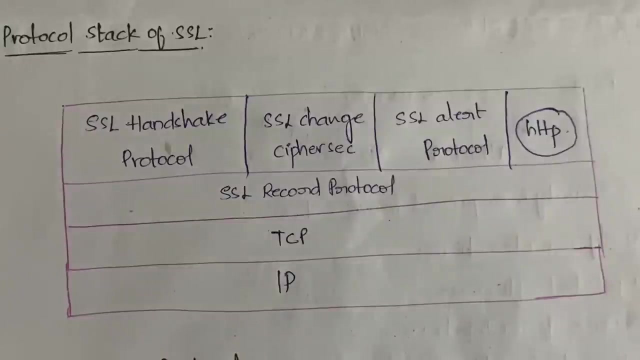 and we also have a http protocol right and again ssl record protocol, tcp and ip got it now. so these, yeah, one more thing i forgot to tell you. i'm not going to explain about http in detail. in the next video i will explain about the http hypertext transfer protocol and why do we use this and all. 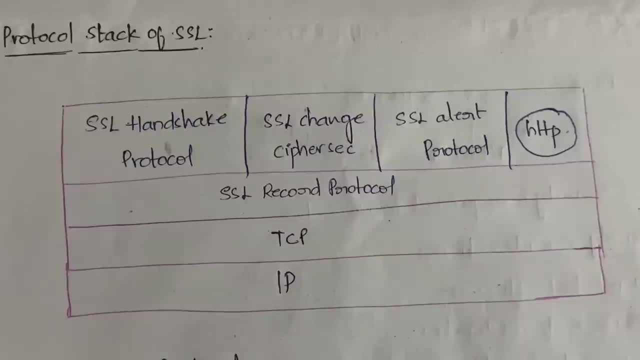 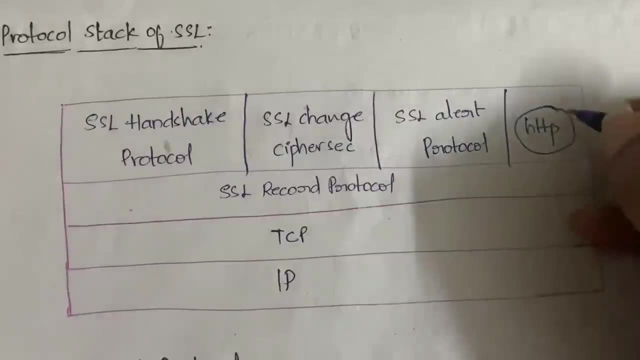 so in the next video i'll explain about the https. so there, i'll just give you a brief overview about the http. as of now, we are not going to discuss about that, because that is very basic for us, right? so this is nothing but normal http. what you know about normal http that you can write? 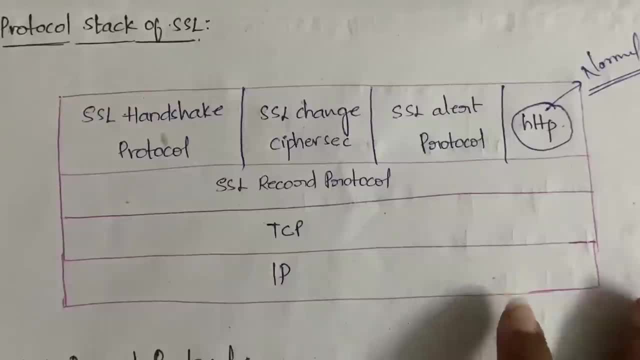 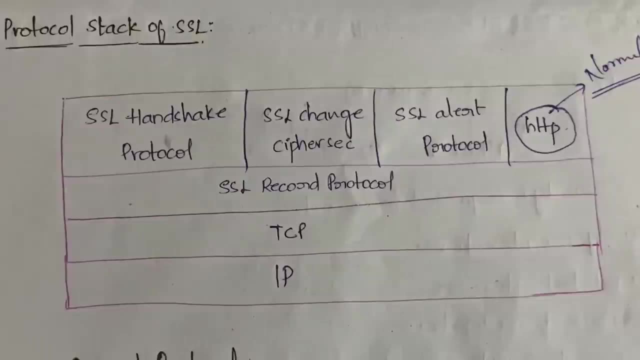 in exam. okay, in exam, if they ask you to write about the ssl protocol, you need to draw this and you need to explain about each and everything. if, in particularly, they asked you about the ssl handshake protocol, you need to elaborate it. otherwise, whatever you know about the ssl protocol, 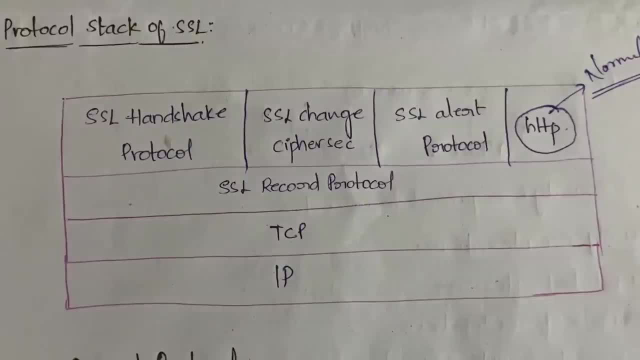 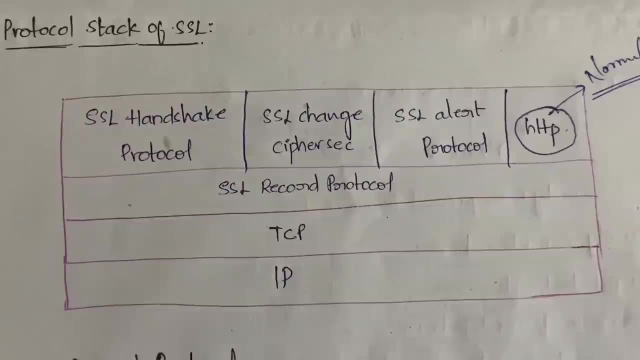 that you can, according to the marks you just elaborate. it got it. so, uh, here in this video, we now. now, what we will learn is we will learn about the ssl record protocol right in the next part of the video. i'll explain all these three, all these three at once. i will explain in the next. 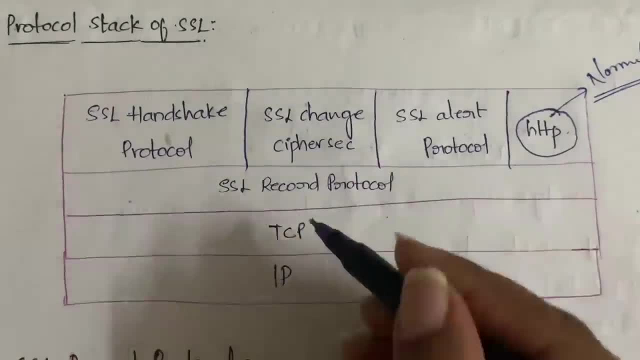 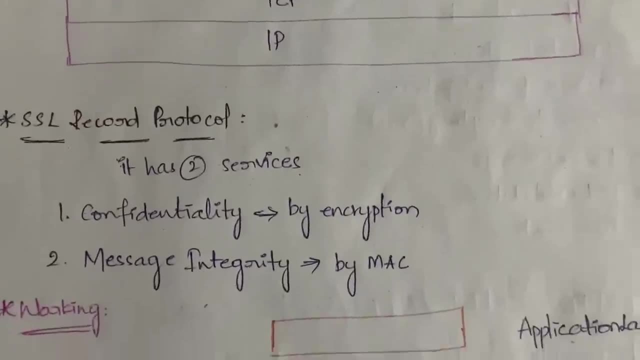 part of the video. for now let us learn as a ssl record protocol and tcp and ip. i'll not explain you separately because you already know tcp and ip in the previous subjects. right, you have learned now ssl record protocol. so basically, ssl record protocol has two services. it provides confidentiality. 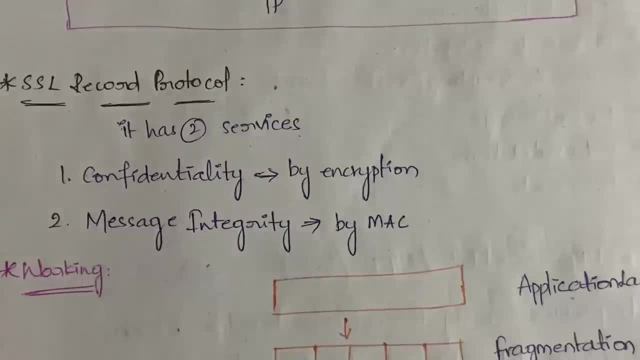 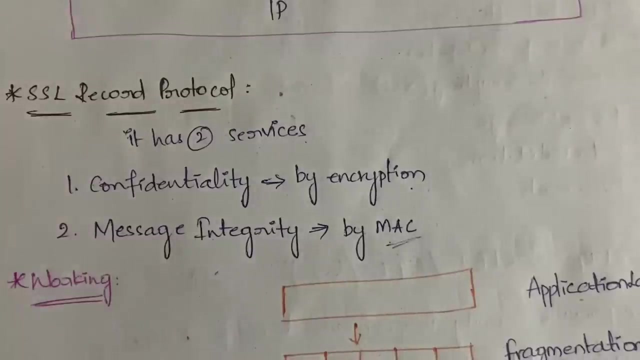 uh data and also it provides the message integrity, that is, the message is not altered. and what do you mean by confidentiality? the message is not known to the third person, right? so confidentiality, you can get it by encryption, and message integrity, you can get it by using mac message authentication code. got it, so it is very easy. i'll explain you with this. 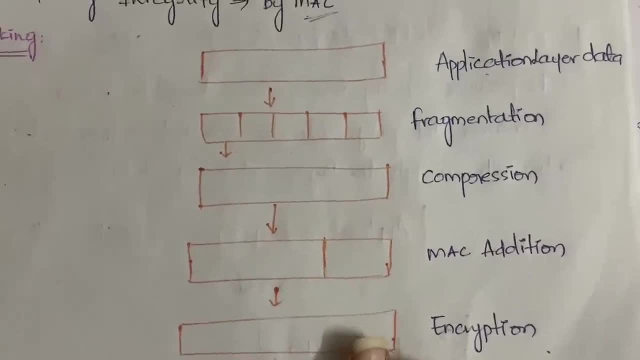 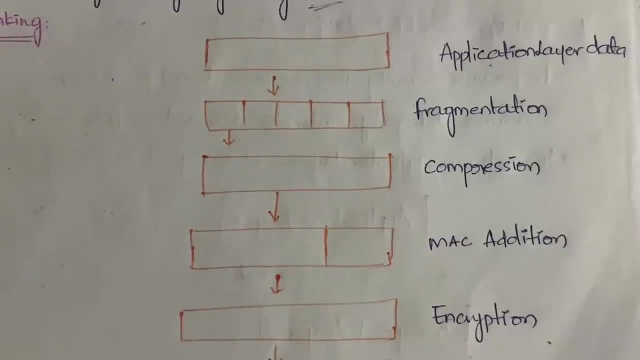 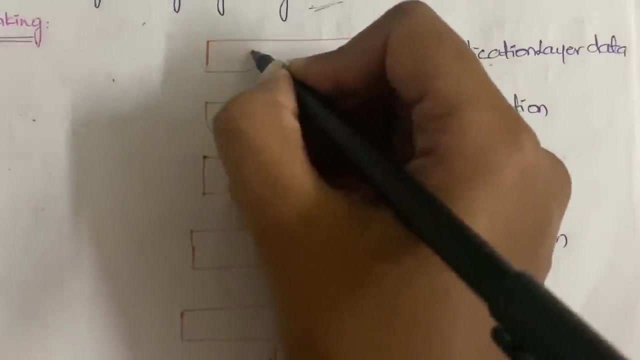 uh, diagram, you know diagram, flow chart, whatever it is. i'll explain you with this. so, basically, when data from application layer is trans, you know when data is coming from the application layer. whatever data is, uh, you is present in the application layer. so this is the data which. 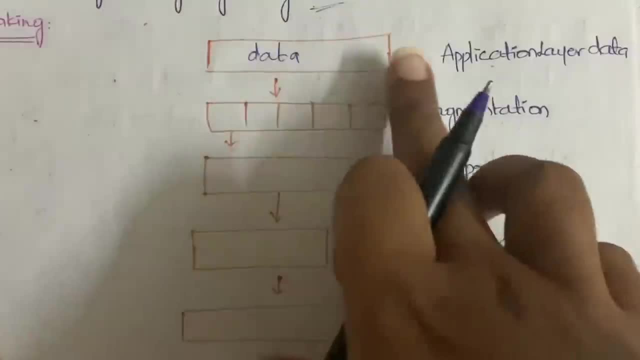 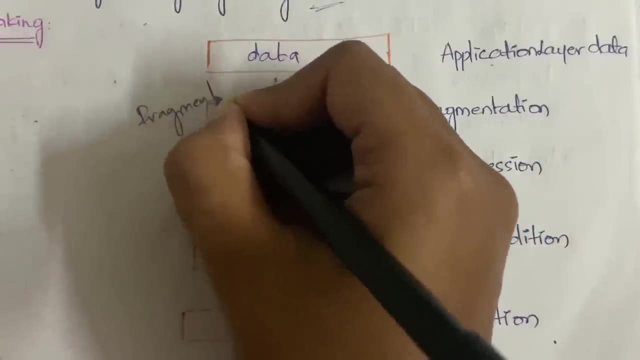 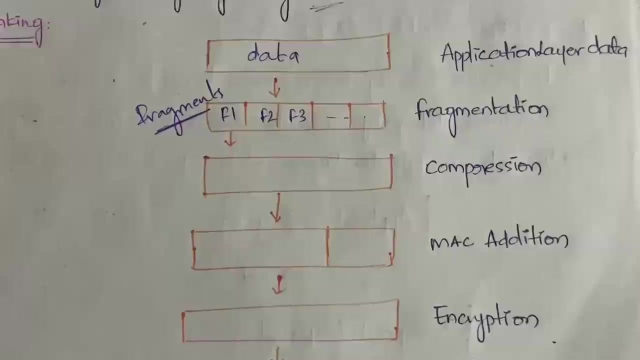 is present in application layer, got it. so the application layer data is divided into number of fragments, right, and that process is called as fragmentation, so it is divided into number of fragments. so this is fragment: one fragment, two fragment, three, like that, based on the size of the 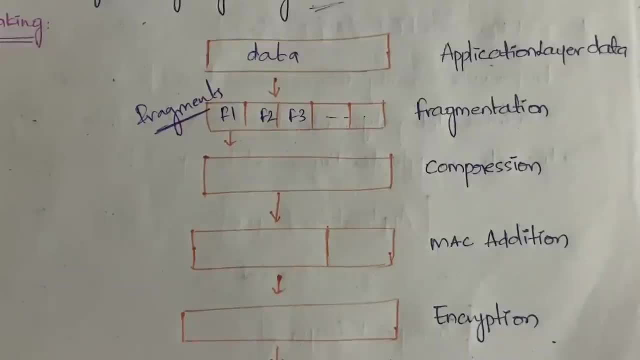 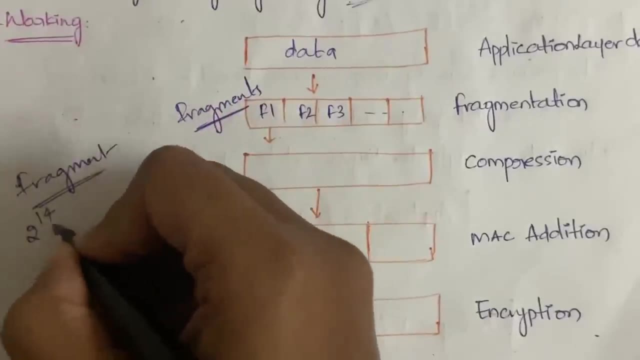 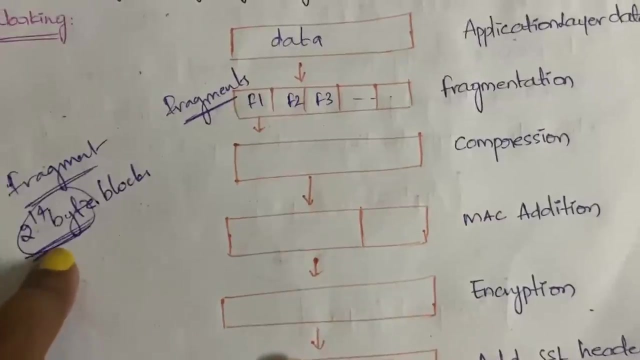 data. it is divided into number of fragments and the size of each fragment will be equal to each fragment. size is nothing but 2 power 14 byte block. so you'll be getting each block of each block with size of 2 power 14, right, based on the data size we will be dividing it into. 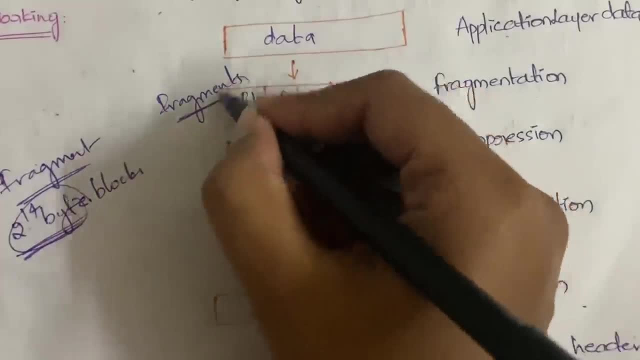 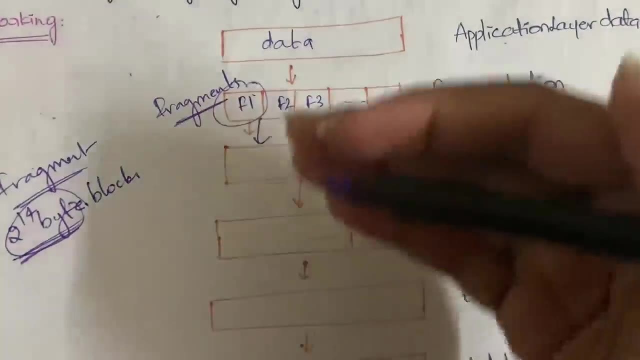 number of fragments. once you divide it into number of fragments, each fragment you will take. so only one fragment you will take. that is only one in the sense, for each and every fragment here onwards, whatever we are going to do, that process will be followed for each and every. 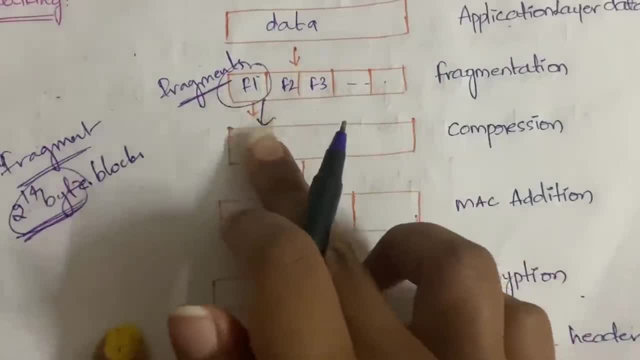 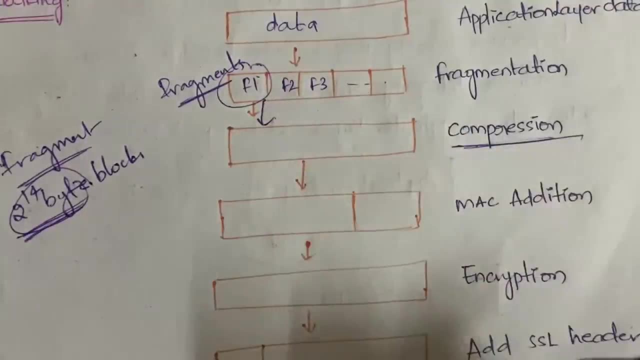 fragment. okay, so you're gonna take one fragment and that for and for that fragment. what you have to do? you need to do the data compression, got it. you know what is data compression? right? you're reducing the size of the data and this compression has to be loss less compression in compression. we 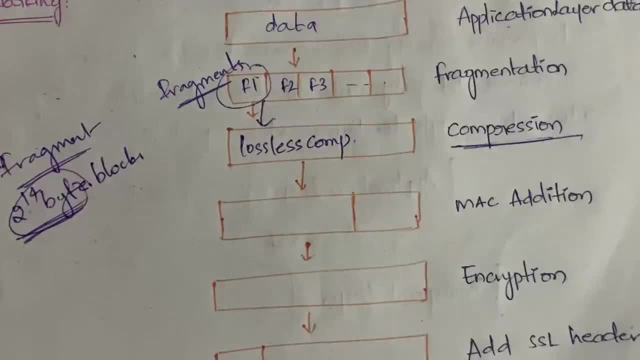 have two types right: lossy compression and loss less compression. in lossy compression, what we're is done. what happens? loss of data happens. some data, some, you know, small data loss can happen. but in case of loss less compression, data loss will not happen. at the same time, the size of the 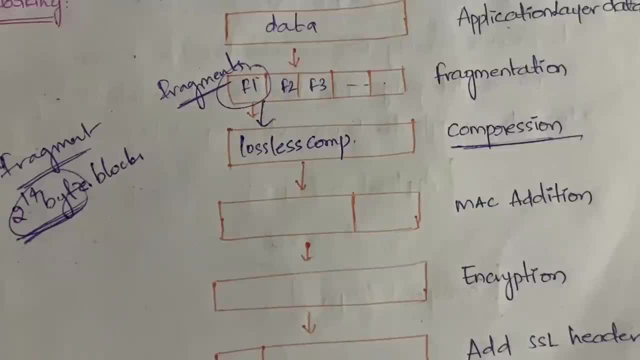 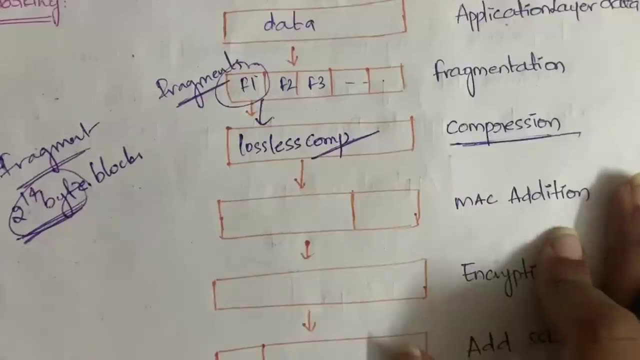 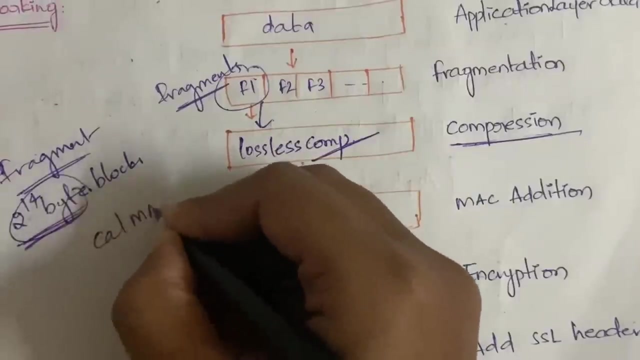 data will be compressed. got it. so this is the loss less compression. so here, whatever compression we are doing, that has to be done. lossless compression has to be done. got it now. after doing the lossless compression, what you have to do is you need to calculate the mac code. got it. so for the data, for: 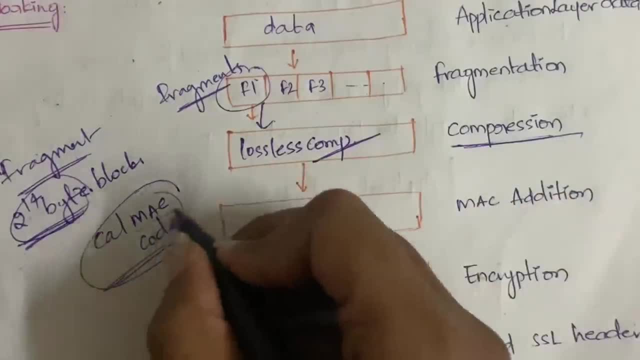 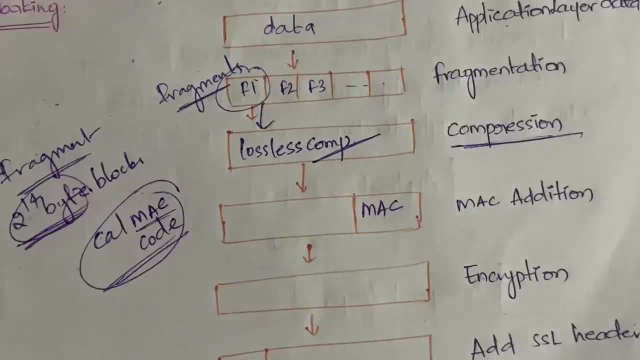 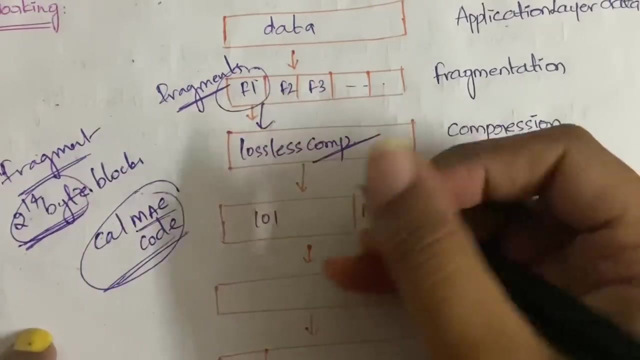 this data, you need to calculate the mac code. once you calculate the mac code, you need to add that mac code at the end of the data, at the uh near the tail of the data. to the end you need to add that macro. for example, our data is 101 and the mac code which we have calculated is 0 0, 1, right. so this? 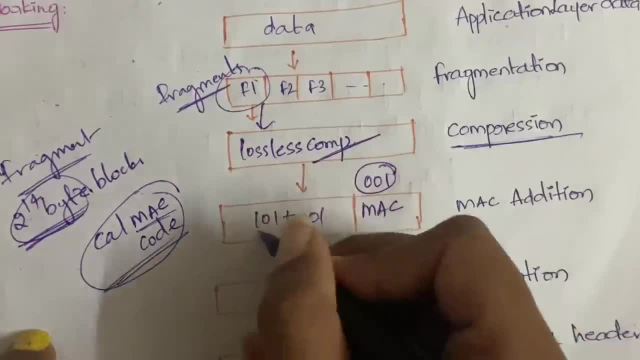 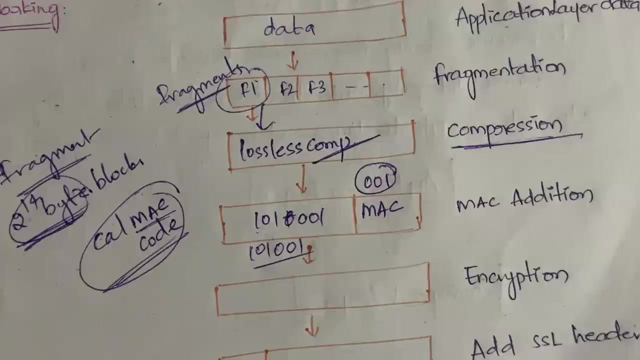 zero, zero. one has to be added to this. this, that is one added in the sense, not exactly addition. you can say append, okay, so it becomes 101001. so you need to attach the mac code generated at the end to the original data, which, whatever you're having done now, mac edition is also done. so once you do the mac edition, 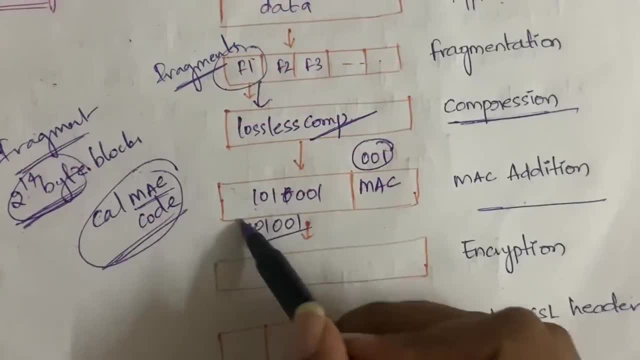 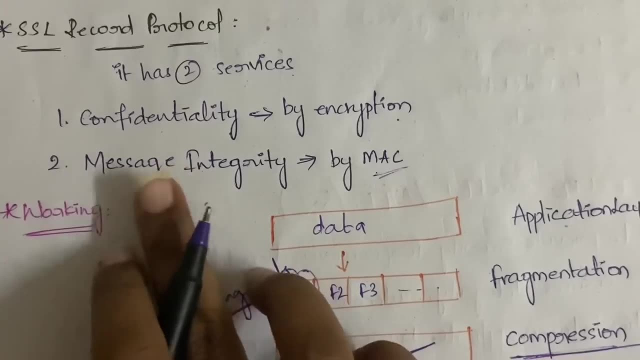 next what you have to do is so for this complete data block again, you need to do the encryption. why encryption and why mac edition? mac edition, we are doing in order to ensure the message integrity and encryption we are doing in order to ensure the confidentiality of the message. 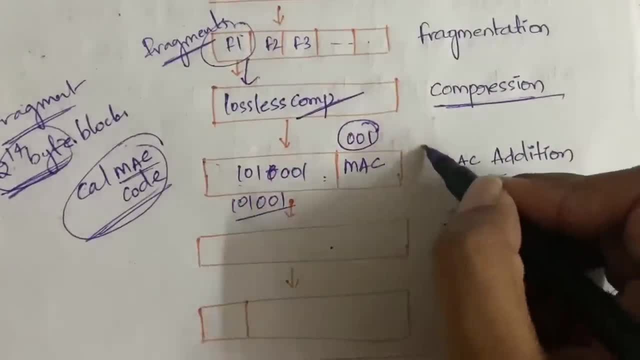 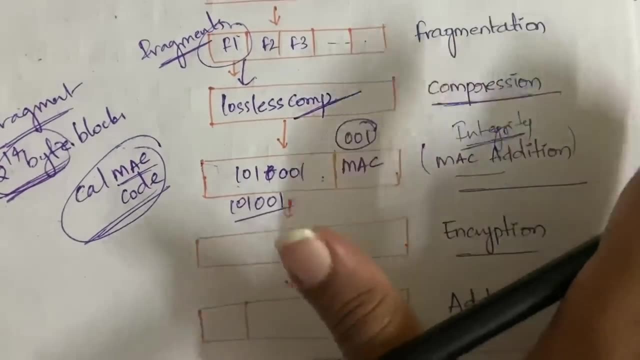 got it. so here what you are doing, mac edition. so in this step you're gonna get message integrity. so we have discussed in the initially what we have discussed in ssl record protocol: we are gonna get confidentiality and message integrity right. so in handshake protocol we will be getting 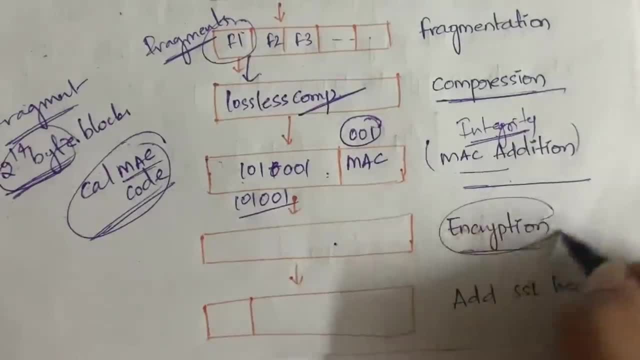 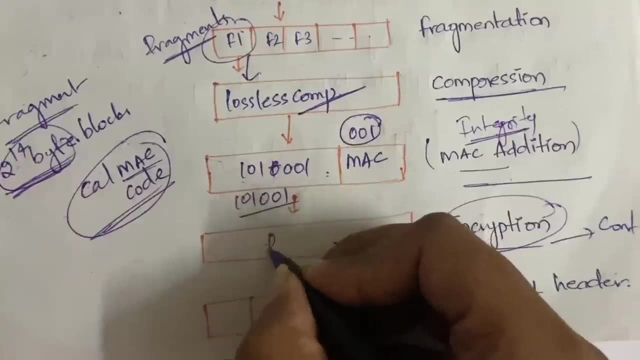 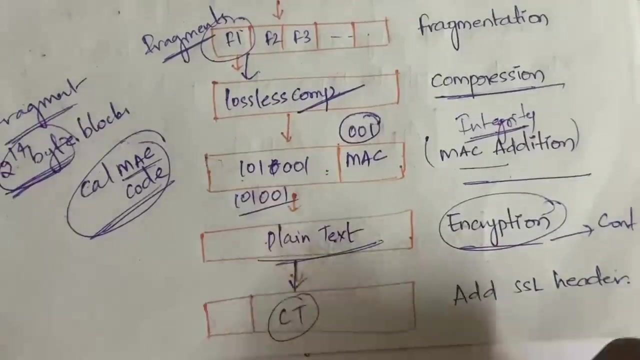 the authentication. and so why do we do encryption, encryption? encryption for the purpose of confidentiality of the message. now, so, before encryption, what we actually call the data, as we call the data as plain text, right? so once you do the encryption, you will be getting the corresponding ciphertext right. so for this ciphertext, that is, 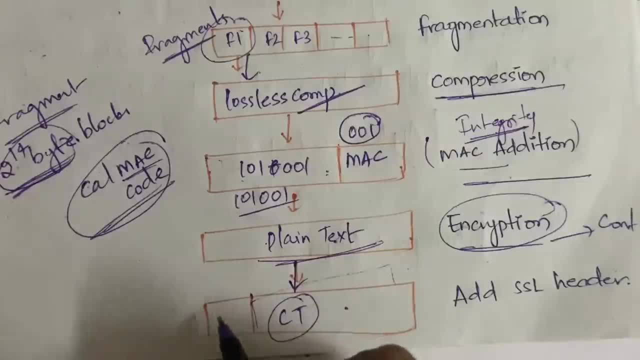 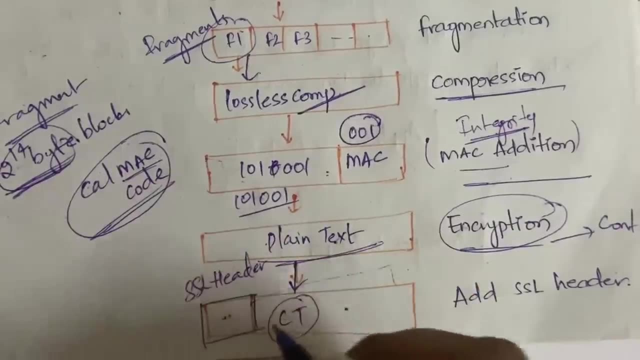 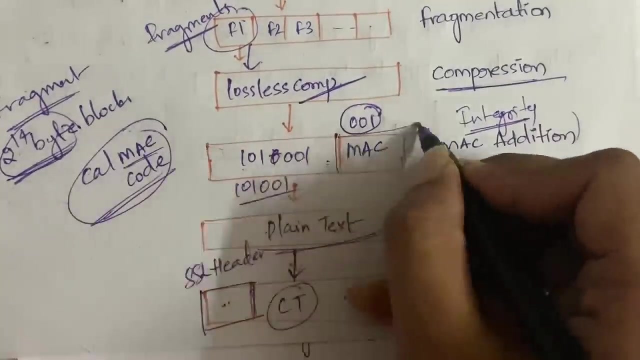 for this encrypted data, you have to add the ssl header. okay, so, ssl header. and where you have to add this ssl header in the start of the, you know, near the head, near in the start of the data that is here you are adding the mac address at the end. right, you are joining the mac address at the end.